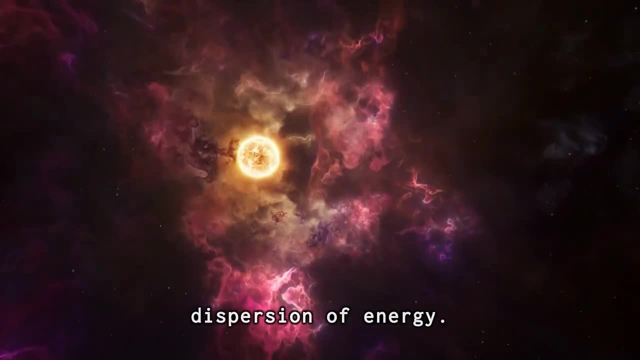 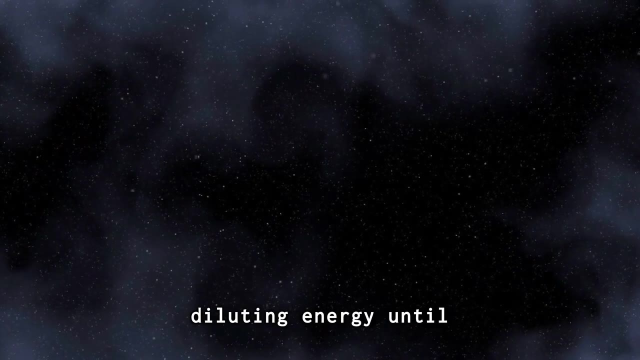 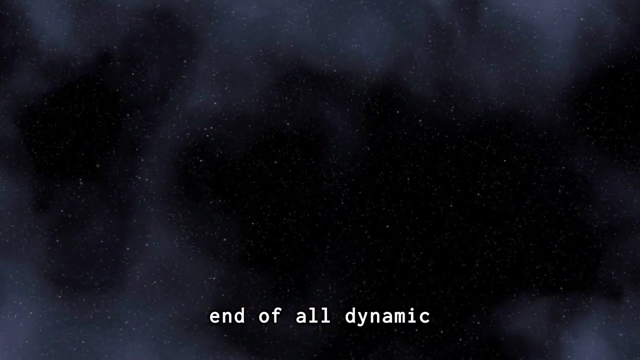 The path to heat death is driven by the gradual dispersion of energy. As stars burn out and galaxies drift apart, the universe expands, diluting energy until it spreads so thin that no work can be performed, signaling the end of all dynamic processes. Another fascinating theory is the Big Rip, where the universe tears itself apart. 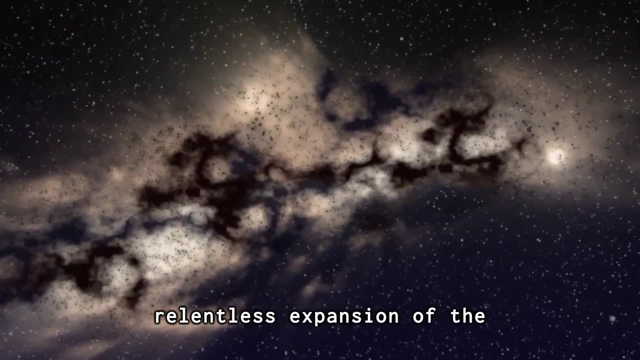 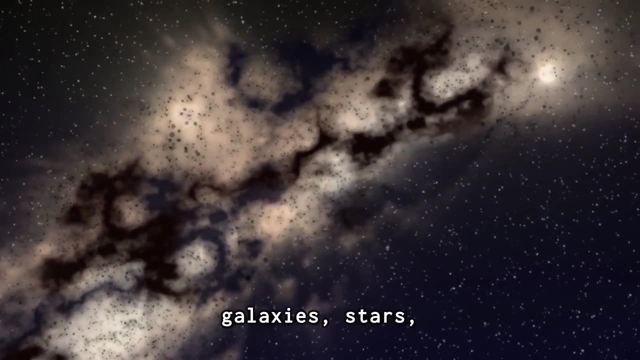 This theory is a theory of the big rip, where the universe tears itself apart. This cataclysmic event is predicated on the relentless expansion of the universe, accelerated by dark energy, As galaxies, stars and, eventually, atoms are ripped asunder. 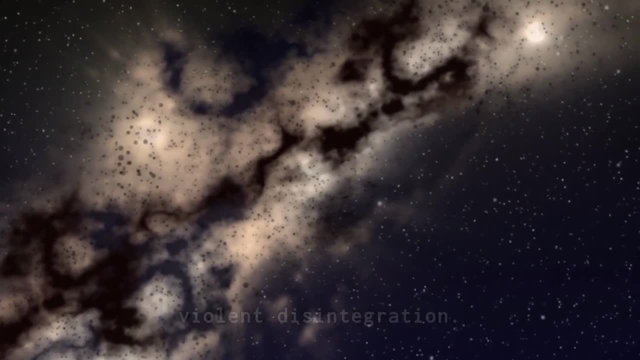 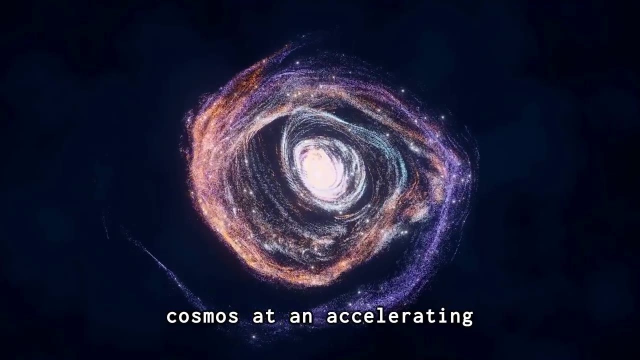 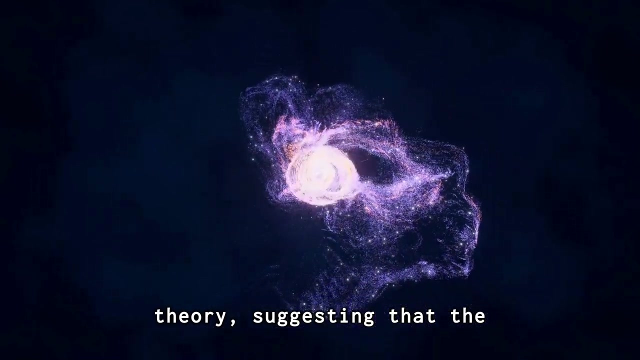 the cosmos faces a violent disintegration. Dark energy remains one of the universe's greatest mysteries, driving the expansion of the cosmos at an accelerating rate. This mysterious force is central to the Big Rip theory, suggesting that the universe is in a state of unhappiness. 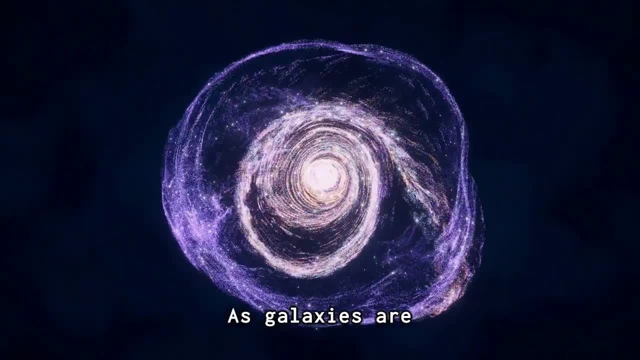 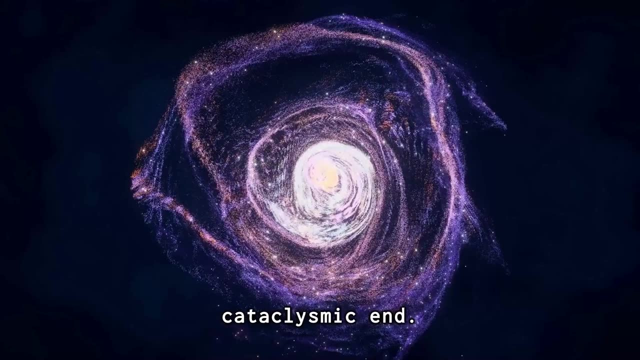 The universe is in a state of unhappiness. The universe is in a state of unhappiness. The universe could eventually be torn apart As galaxies are propelled away from each other. the fabric of the universe stretches beyond its limits, leading to a cataclysmic end. 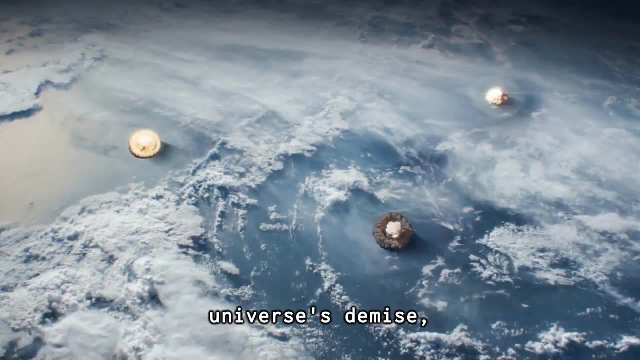 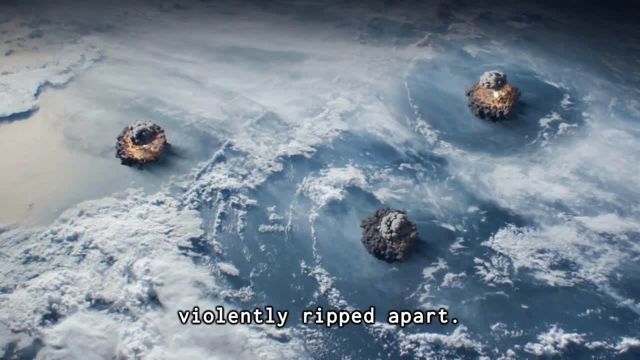 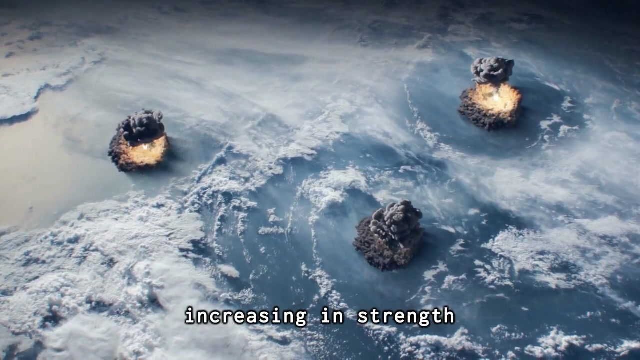 The Big Rip theory paints a dramatic picture of the universe's demise, where not just galaxies but stars, planets and even atomic particles are violently ripped apart. This scenario hinges on the behavior of dark energy increasing in strength until it overwhelms the universe. This scenario hinges on the behavior of dark energy increasing in strength until it overwhelms the universe. This scenario hinges on the behavior of dark energy increasing in strength until it overwhelms all other forces in the universe. increasing in strength until it overwhelms all other forces in the universe. 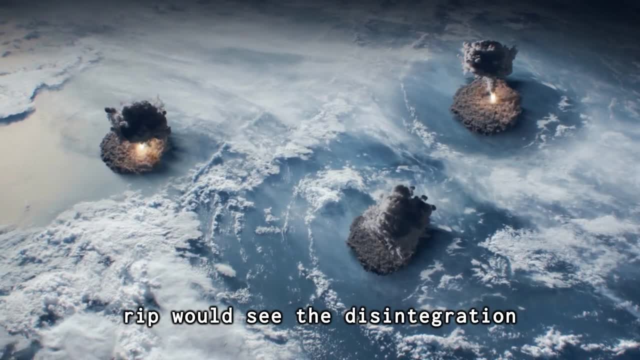 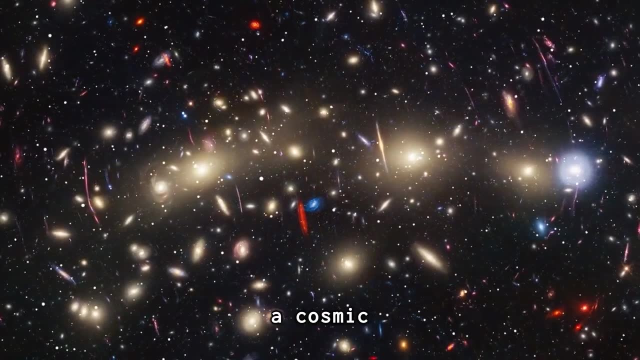 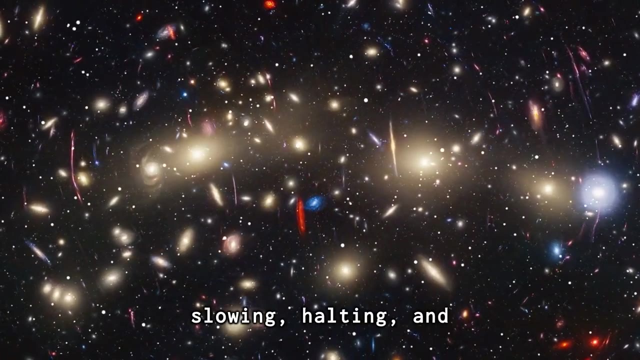 The final moments before the rip would see the disintegration of everything we know. Conversely, the Big Crunch theory offers a contrasting end: a cosmic collapse. This theory envisages the universe's expansion slowing, halting and eventually reversing, leading all matter to crash back into a singular point. 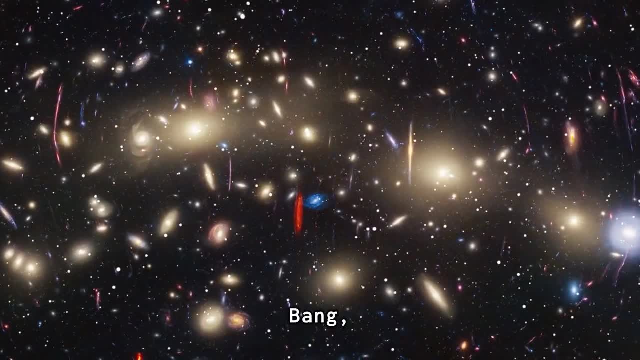 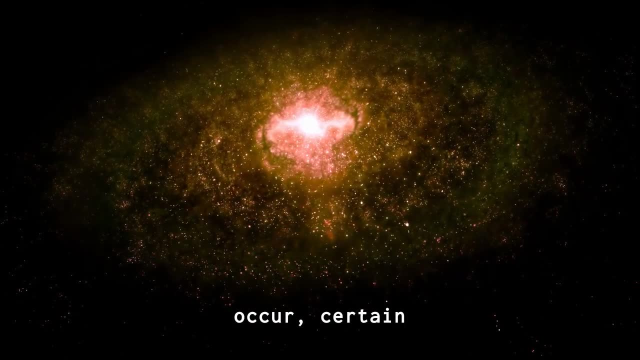 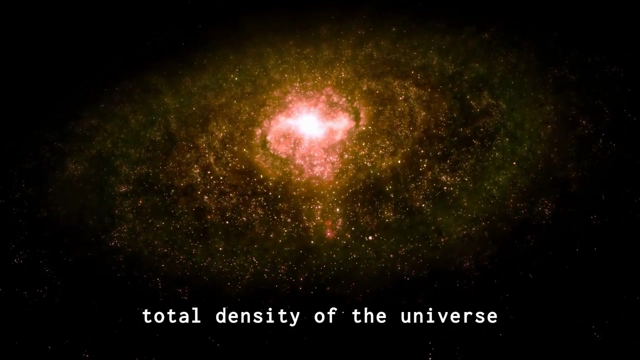 This scenario would effectively reverse the Big Bang, culminating in a universe that implodes rather than expands. For the Big Crunch to occur, certain conditions must be met, primarily related to the universe's density. If the total density of the universe is above a critical level, 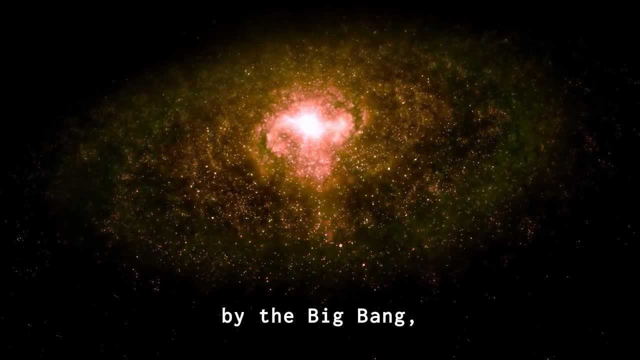 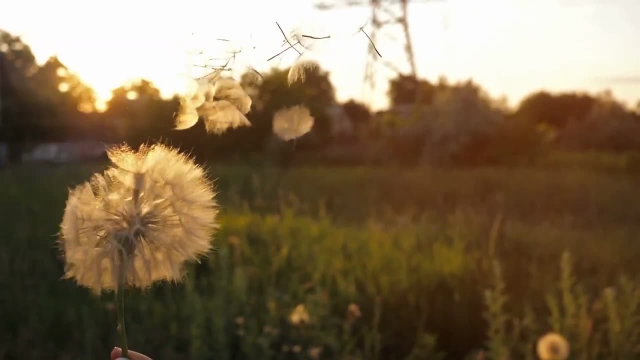 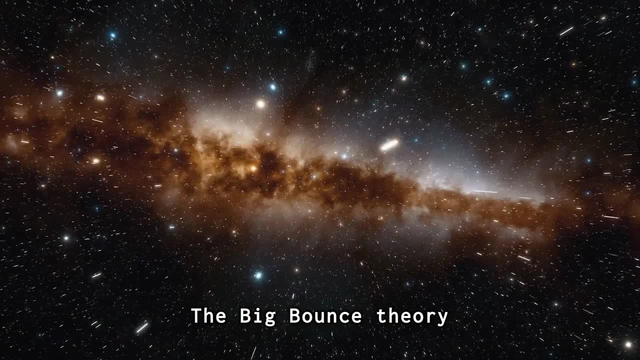 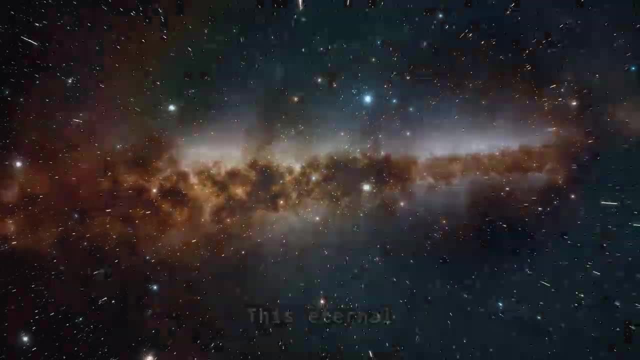 Just hang on, Just hang on, Just hang on. It's a bit depressing, but we are almost done. The Big Bounce theory proposes a cyclical universe, suggesting that each Big Crunch could be followed by another Big Bang. This eternal cosmic cycle implies that our universe might be one of many. 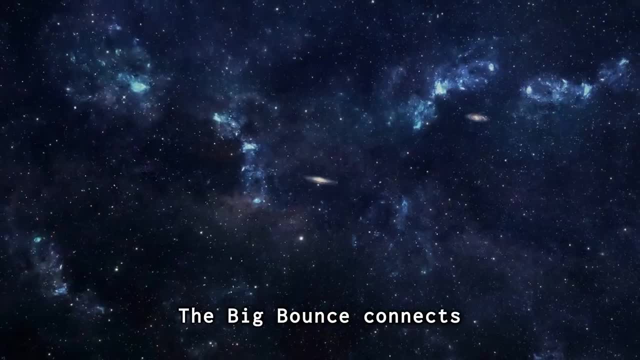 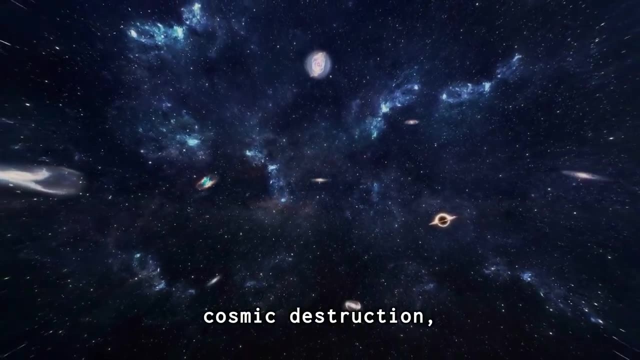 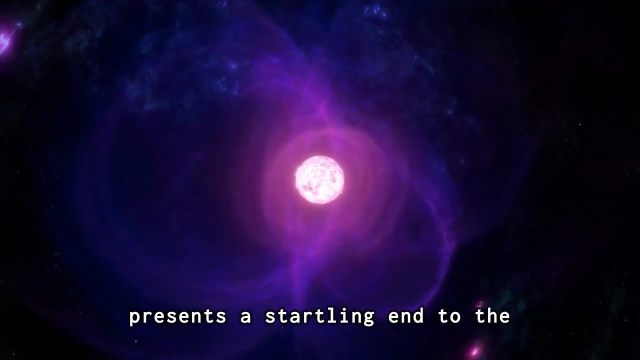 in an infinite series of universes. The Big Bounce connects directly to the Big Crunch, offering a glimmer of renewal amidst cosmic destruction, hinting at a universe that is eternally reborn. The Big Slurp, or vacuum decay, presents a startling end to the universe rooted in the instability of the quantum. 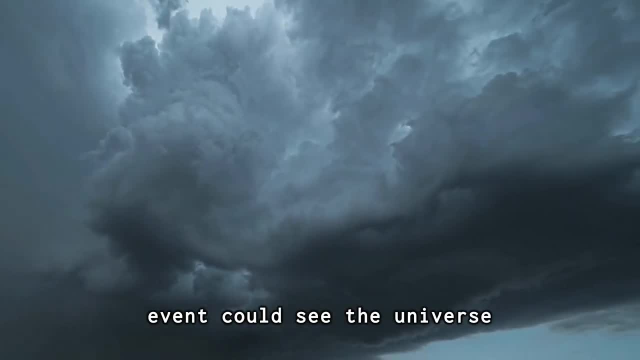 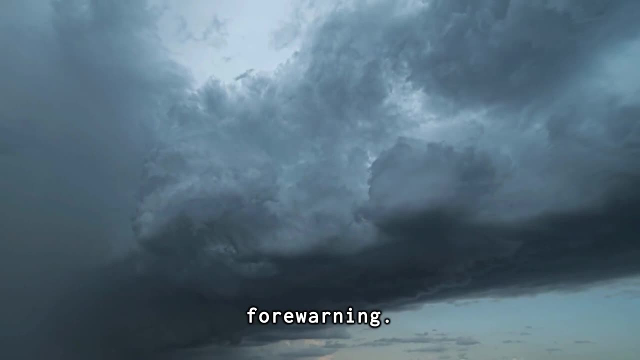 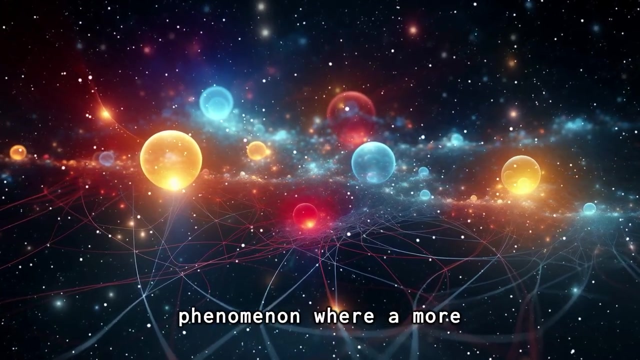 field. This cataclysmic event could see the universe collapsing into a more stable vacuum state, eradicating everything instantly without any forewarning. Quantum fluctuations serve as the catalyst for the universe's big slurp, a phenomenon where a more stable vacuum state 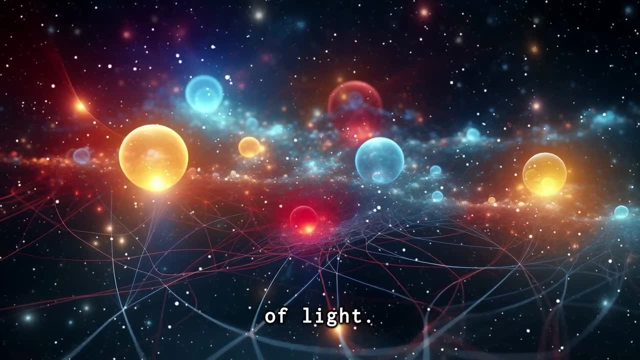 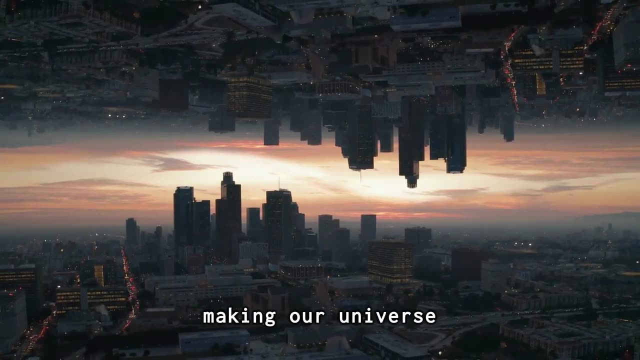 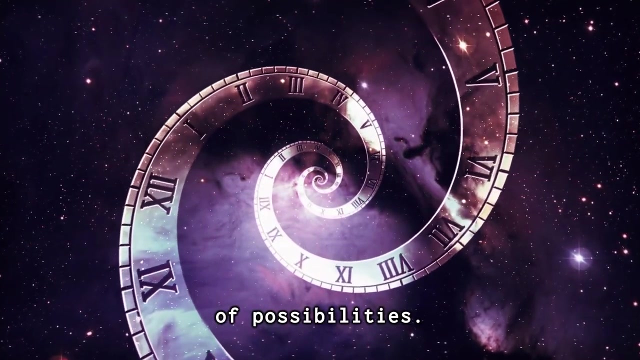 bubbles through our current universe at the speed of light. This transition would fundamentally alter the fabric of reality, making our universe unrecognizable. Comparing the timelines of these cosmic events reveals a vast range of possibilities, While some theories suggest an imminent end. 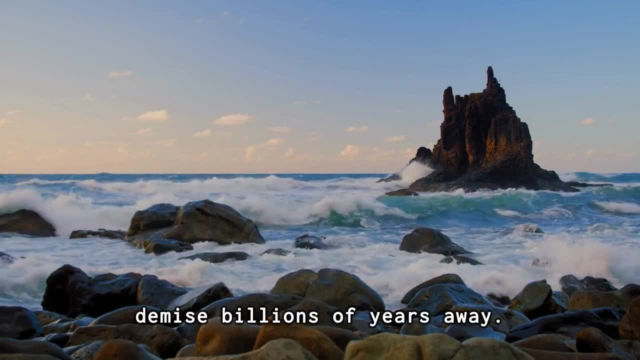 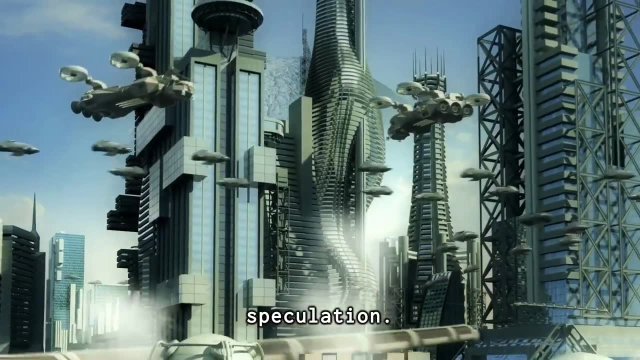 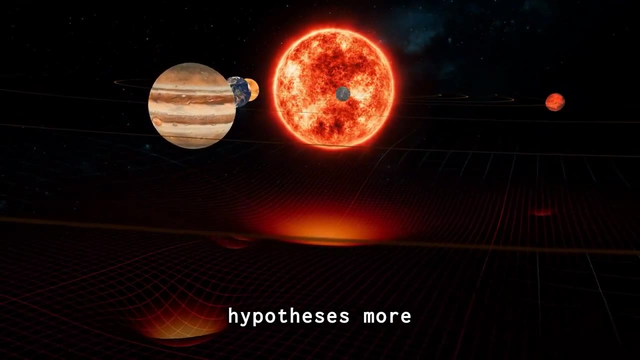 others propose a demise billions of years away, The uncertainty underscores the unpredictability of cosmic fate, leaving much to speculate. The scientific evidence supporting each end of the universe theory varies widely, with some hypotheses more grounded in observational data than others. Researchers rely on advanced simulations. 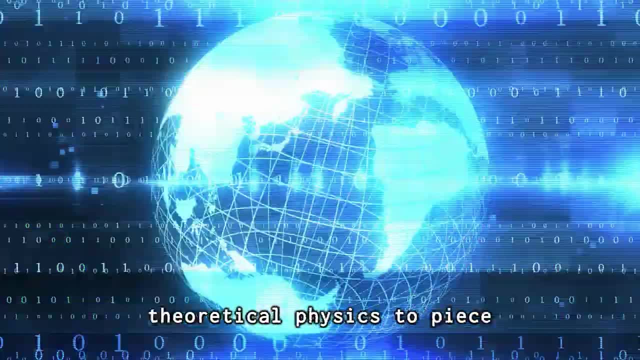 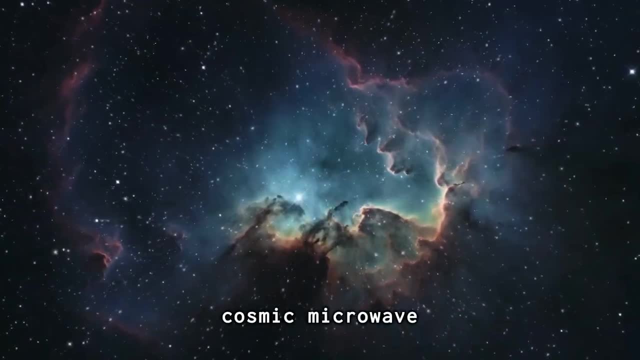 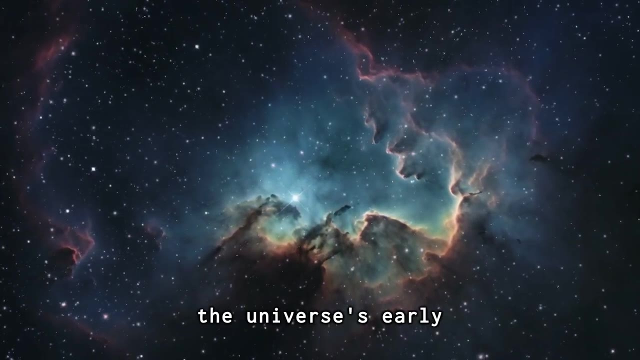 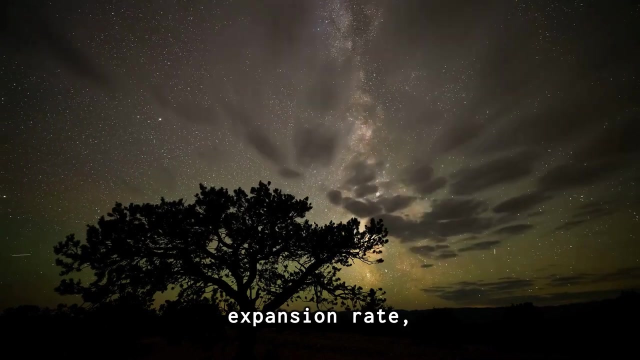 astronomical observations and theoretical physics to piece together the possible fates awaiting the cosmos. Observations of the cosmic microwave background, CMB, offer crucial insights into these theories. By studying the CMB, scientists can infer the universe's expansion rate composition. 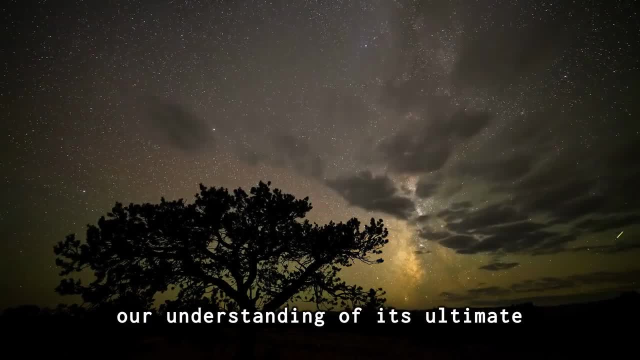 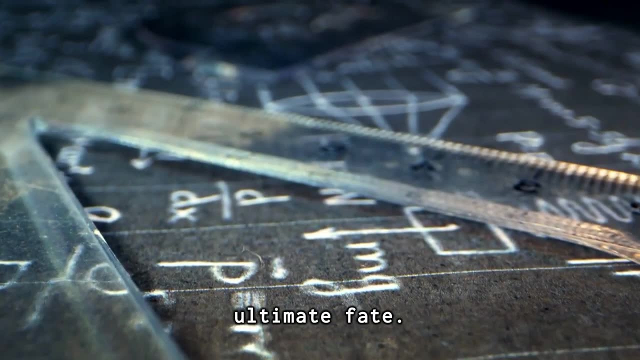 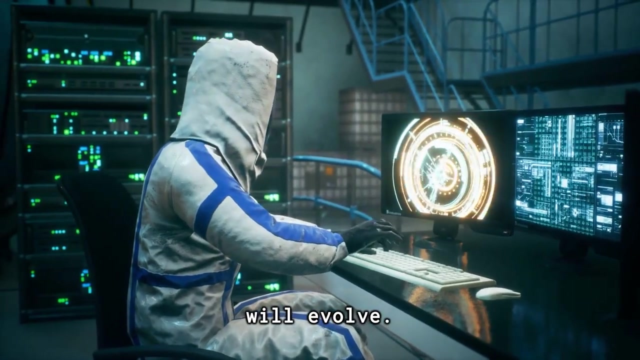 and potential destiny, shaping our understanding of its ultimate fate. Particle physics plays a pivotal role in deciphering the universe's ultimate fate. By understanding the fundamental particles and forces, scientists can predict how the universe will evolve. This field is crucial for testing science.